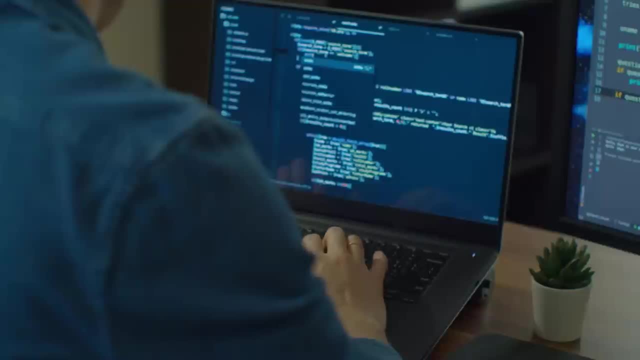 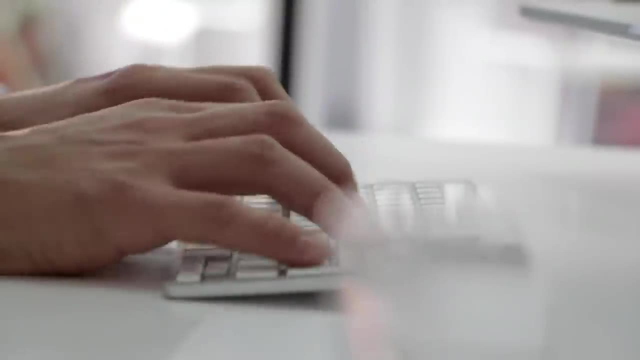 which allow you to build reusable standalone custom HTML elements. These components are no different than the usual components you might be used to when working with libraries like React or Angular. They have their own behavior written in JavaScript. they are styled using scoped CSS. 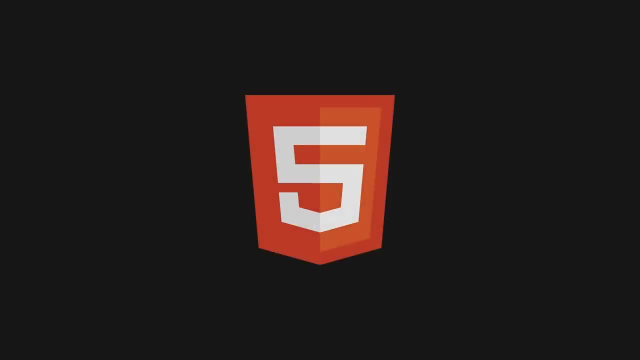 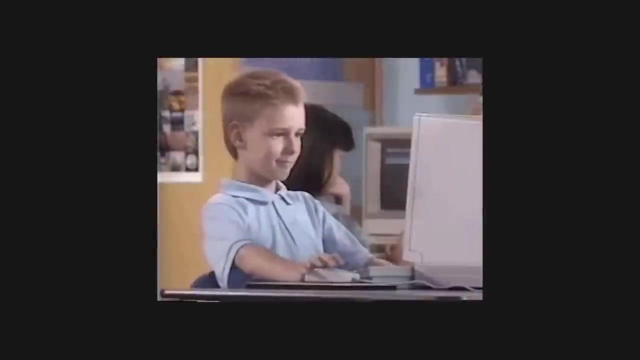 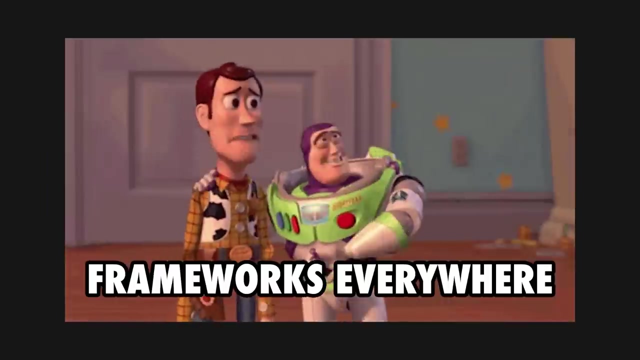 and they use HTML and string interpolation for templating purposes. Even though the developer experience might be a tad different, with Web Components you'll be able to build the same type of reactive, powerful user interfaces all modern web apps are providing. Why use Web Components in favor of one of the many other established solutions? 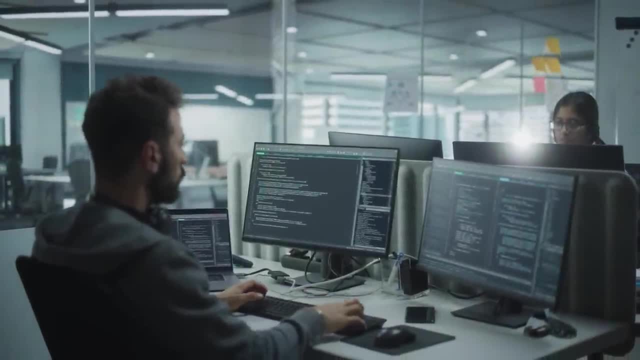 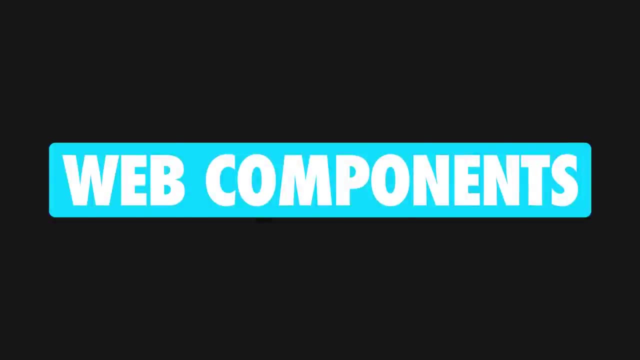 First of all, your code will only rely on web standards. This means little to no JavaScript overhead sent over the wire. There is no framework, internal logic or third-party hidden dependencies, which is more than useful in this day and age when everybody is focusing. 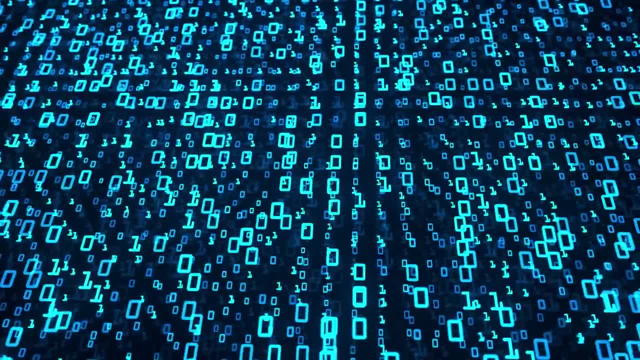 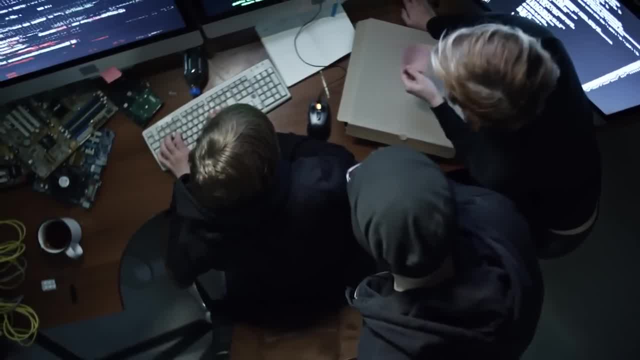 on over-the-wire performance and optimized resource consumption. Second of all, your code will be framework agnostic. Components can be easily reused in other codebases and they will play nicely with any other framework, if that's a requirement. Finally, you'll end up building truly reusable components. In my experience, this is rarely the case when working with React, for instance. You really need to apply yourself to create standalone, isolated components there, but Web Components kind of force you to tackle things in a different manner. Okay, enough with the sales pitch for Web Components. 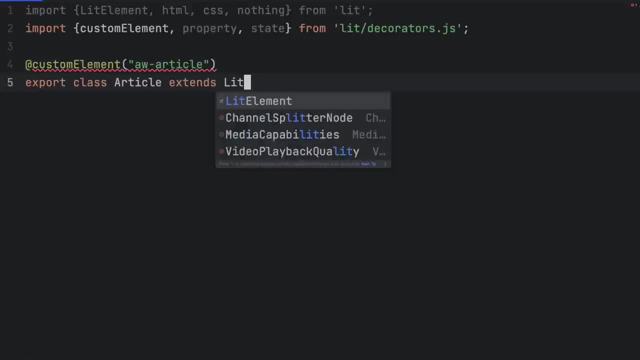 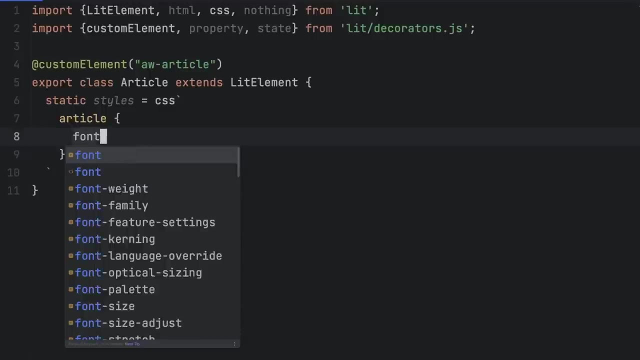 The topic of this video is actually Leet, a lightweight tool that simplifies the way you build Web Components. They just announced their future version 3 release, so this is as good a time as any to take a quick look at the whole Web Components space through the Leet lens. 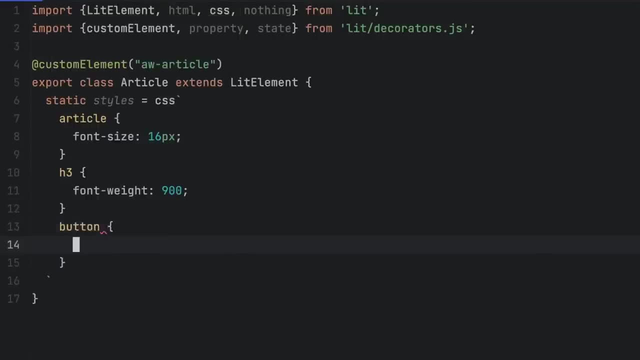 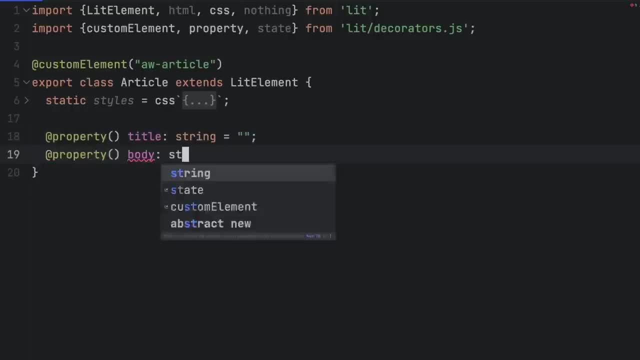 First of all, it is simple, providing a straightforward reactivity model, declarative templates and a handful of other thoughtful features aimed to reduce the boilerplate code. It is also fast, with a tiny footprint: It weighs in around 5KB minified. 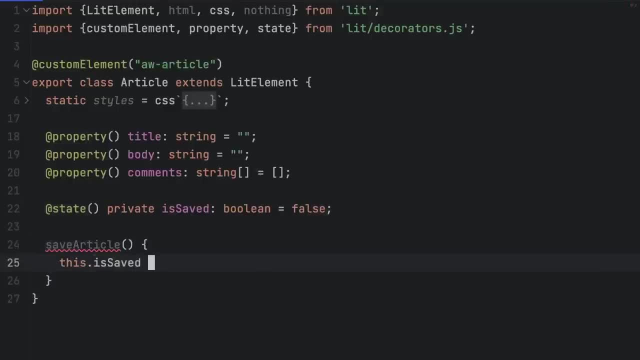 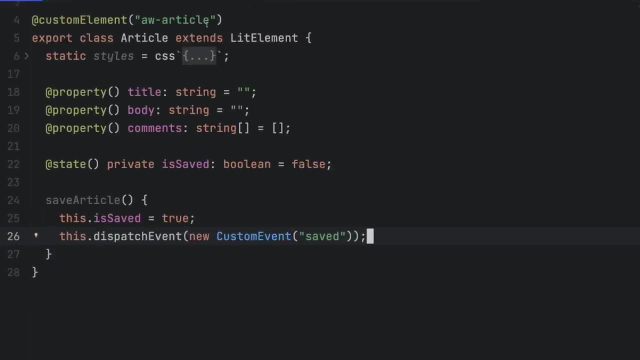 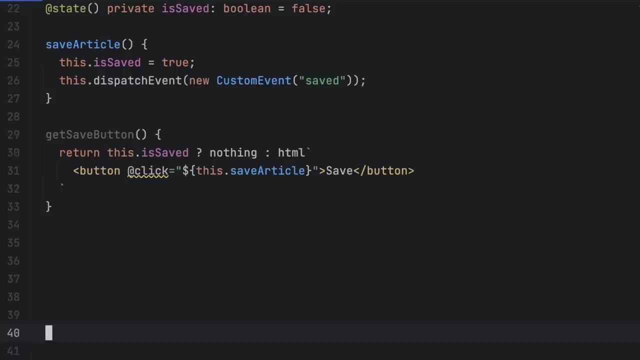 and compressed. It follows the more modern approach of updating the DOM directly when any dynamic part is changing. In comparison, frameworks like Angular, React or Vue are using a virtual DOM diffing strategy, which affects both the complexity of the code and the used memory. Finally, it plays really well with TypeScript, which is always a plus. these 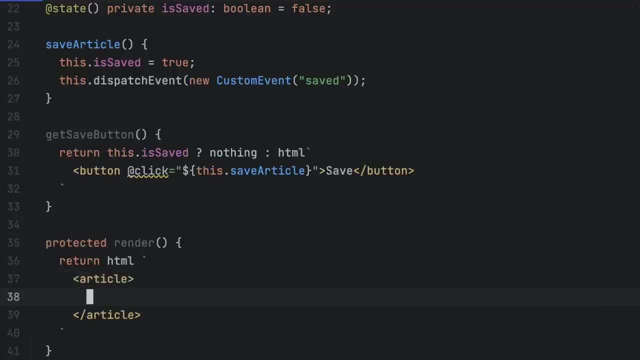 days, since TS is pretty much the norm in front-end development, Despite it not being one of the popular kids. a lot of big established companies are using Leet in production to build shareable component libraries, design systems or even in their websites. 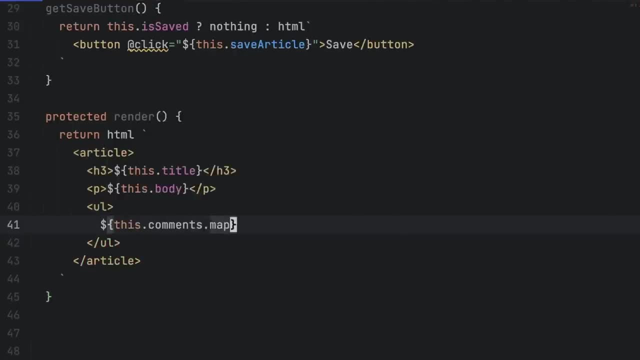 Okay, now let's take a look at a component I built for the past minute or so. Of course, I'm using TypeScript, which allows me to define Leet elements using decorators. Leet components are standard custom elements, so the browsers will treat them exactly. 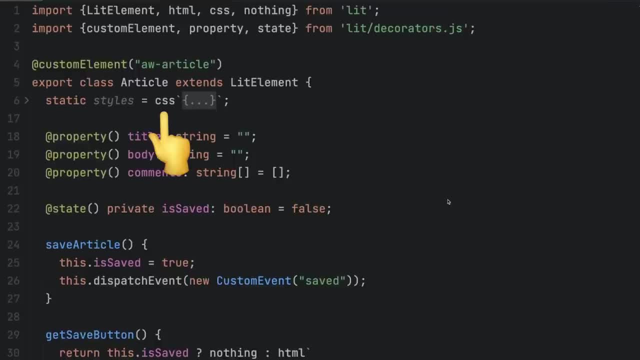 like any other built-in element. Then, using the CSS helper, I can define scoped styling rules for my component. Note that you have to assign the rules to a static styles class property, and Leet will take care of the rest. Next let's take a look at state and props. 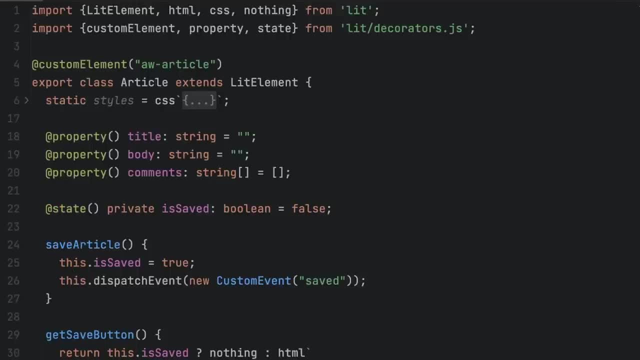 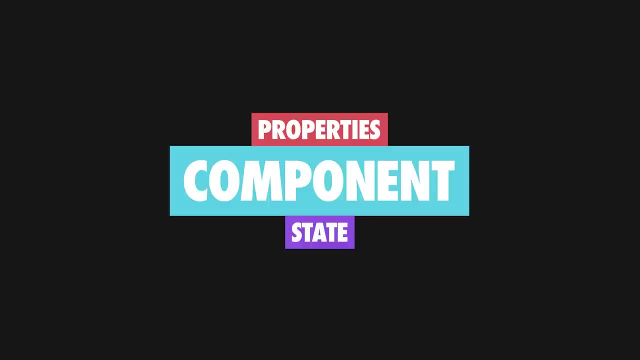 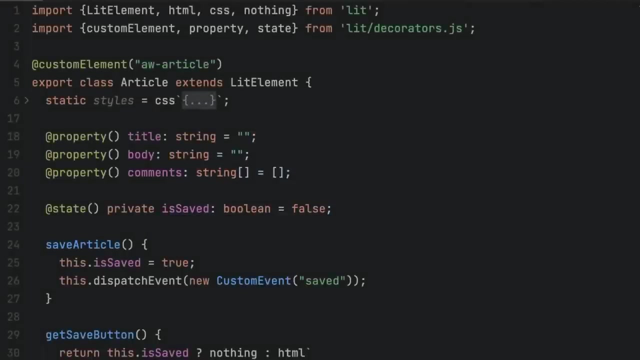 the main actors behind Leet's reactivity. Just like in any other framework, via properties, your component will receive information from the outside world and via state, it'll keep track of the internal data your component needs to handle its business logic. Any change in these fields will cause an update in the render function. 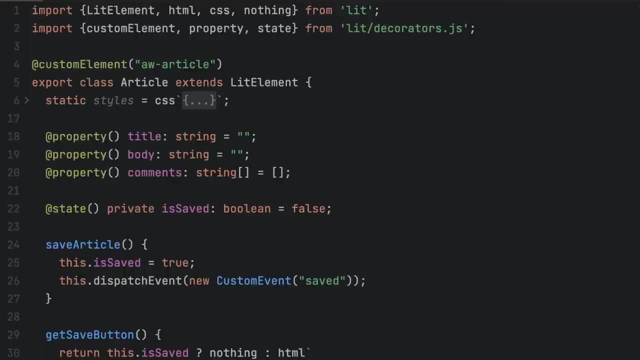 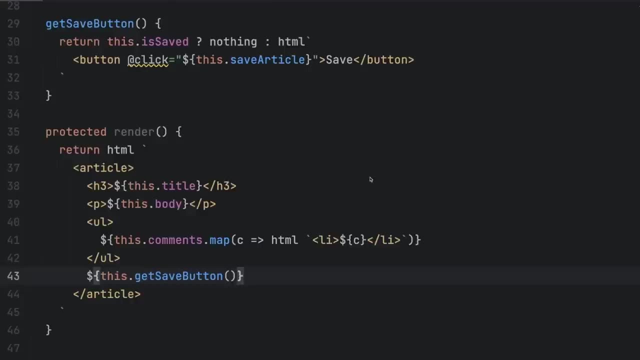 And since I mentioned the world outside your component, you can also send information to parent components via events. Finally, the render function contains the HTML template which will be displayed in the DOM. This implementation is based on template literals and you have full flexibility in the HTML helpers, with support for conditional rendering. 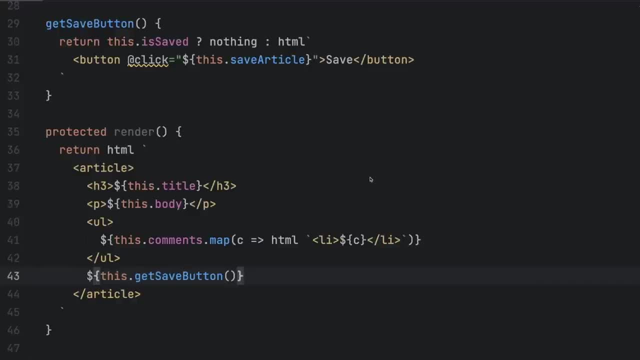 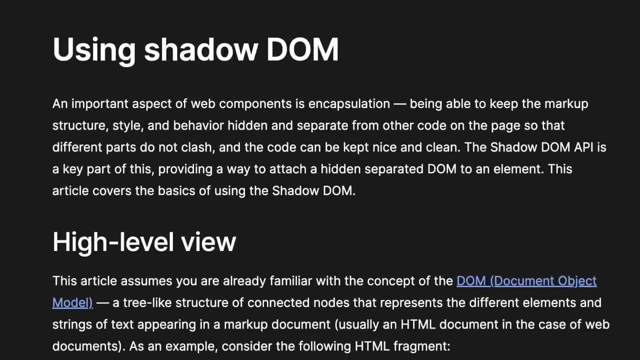 rendering lists and various built-in directives Pretty straightforward, right. Of course, the element in your component DOM can trigger events, and you can either handle those events internally or bubble them up to the outside world. We should also briefly touch on the shadow DOM topic, since this is the mechanism that allows Leet components to add. 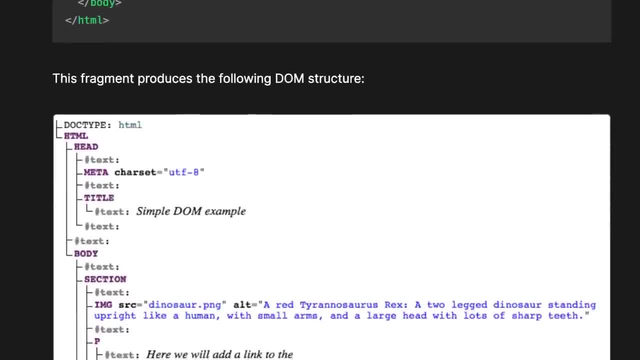 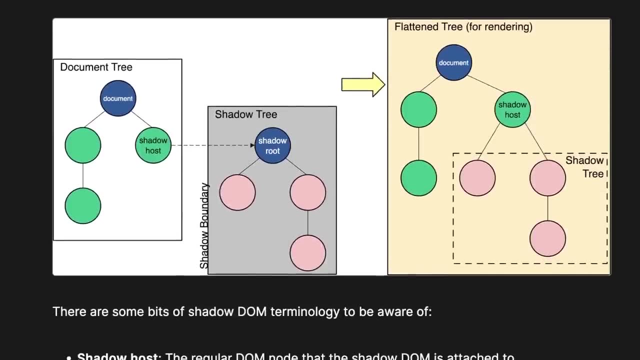 an isolated and encapsulated DOM tree to an element. This approach has two main benefits: DOM scoping, which means that the main DOM won't directly find elements in your component's shadow DOM, so it's going to be harder for global scripts to break your component And style scoping.